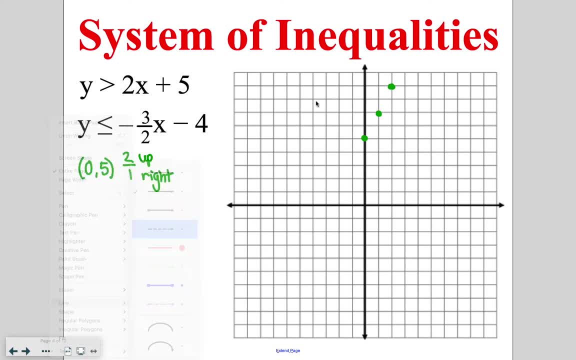 than so there is no equal to part. So I'm going to pull up my y intercept, which is 0- 5, and my slope, which is 2 over 1.. So I'm going to put a dashed line on my graph as I graph this particular. 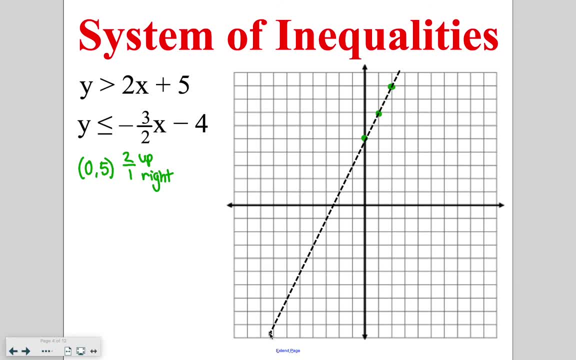 inequality and I want to make sure that I get that as straight as possible. Then I need to go through and I need to do a test point for this graph. So once again, I like to pick 0- 0.. So I'm going to go: 0 is greater than 2 times 0 plus 5, giving me the statement that 0 is greater than 0. 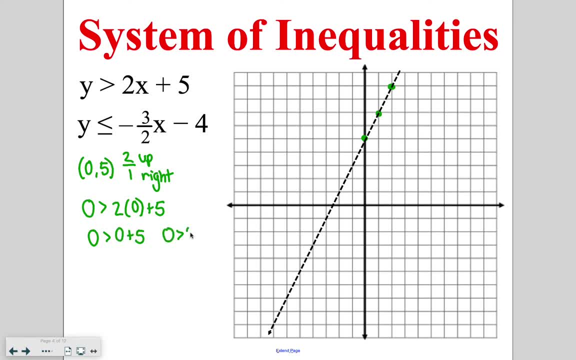 plus 5.. Or 0 is greater than 5, which is a false statement. So 0, 0 is not included in this graph, So I'm going to go ahead and shade the opposite side then. So everything to the left of this line is going to be. 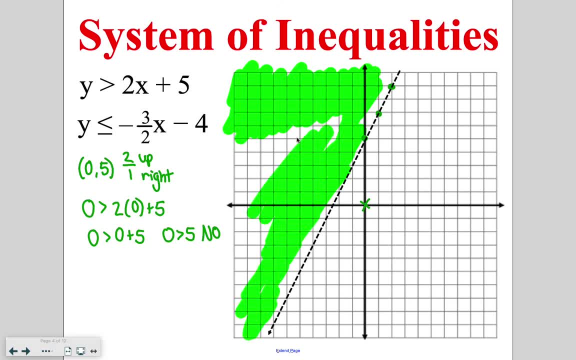 part of my solution for the first inequality. So everything over on this side is going to be part of my solution. Then I need to repeat this process with my second inequality. So I'm going to pick out my y intercept at 0, negative, 4, and pick out my slope which is at negative, 3, 2, which is going to be down 3 and right 2.. So I'm 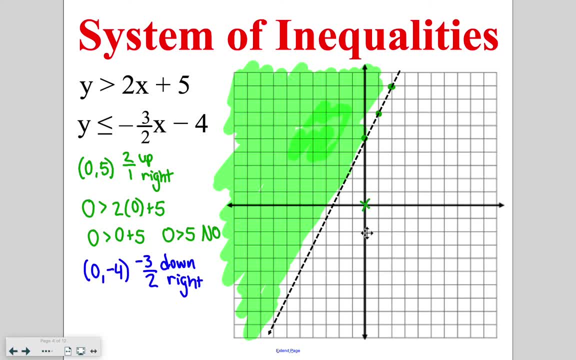 going to put my y intercept at 0, 1, 2, 3, negative, 4.. And then I'm going to go down 1, 2, 3 and right, 1, 2.. And I can do that again: down, 3 and right, 2.. This time my inequality has the equal sign. So I'm going to put a solid line. 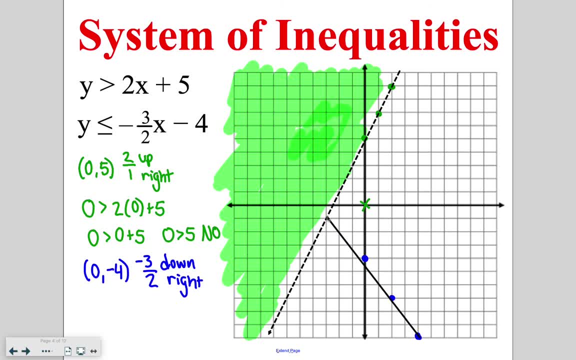 onto my graph as I graph this problem, And I want to make sure I am going all the way through the entirety of my graph when I place that line. so let me just straighten that out just a tad. and that is our second line. now, once again, we need to put a test point in, so I'm going to use zero, zero again. so that's going. 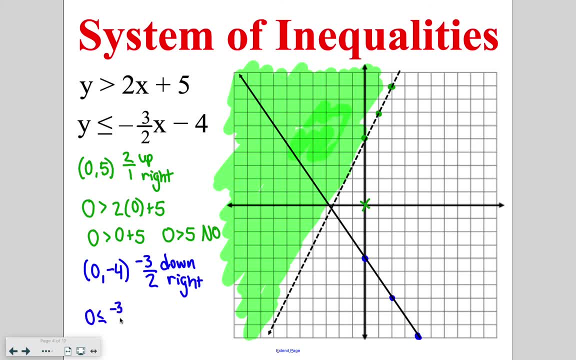 to be. zero is less than or equal to negative three halves times zero minus four. giving me that zero is less than or equal to zero minus four. giving me a final statement of zero is less than or equal to negative four, that is also a false statement. so once again, zero. zero is not part of my solution. 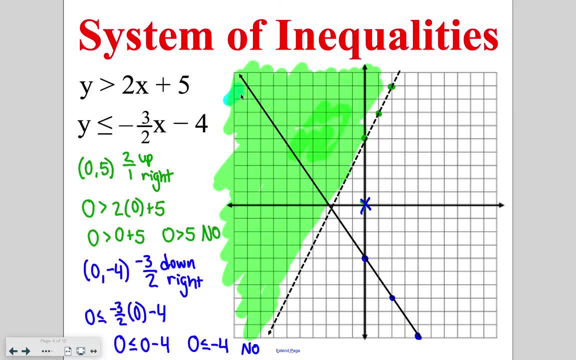 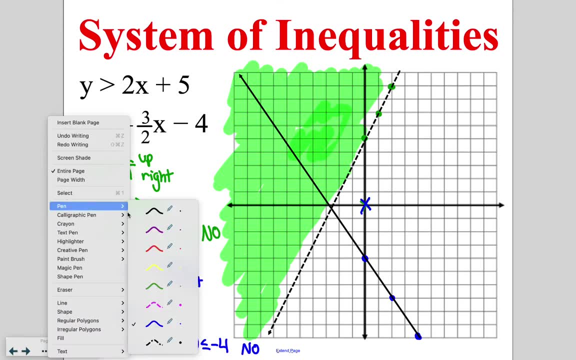 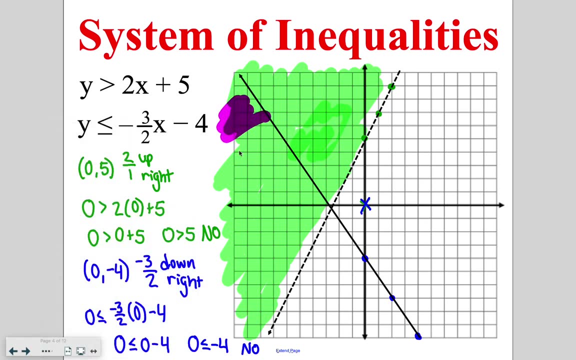 so I'm going to go ahead and highlight in the other side of my inequality, and that's a little bit hard to see. so I'm going to switch colors quickly and I'm going to use zero this purple highlighter instead, so that you can see it a little bit better. 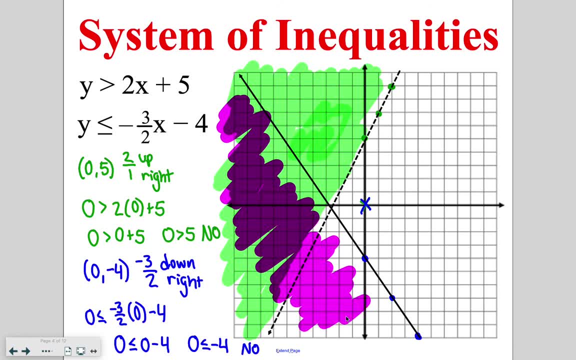 so I've got this side of my graph. now, when we are looking for the solution to a system of inequalities, we are looking for the part of the graph that overlaps. so you have two options at this point. your first option is to take a third color and make it darker. 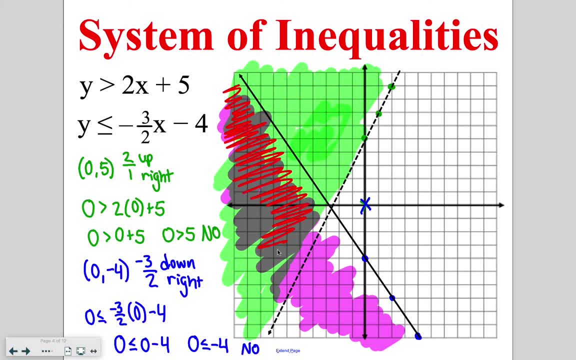 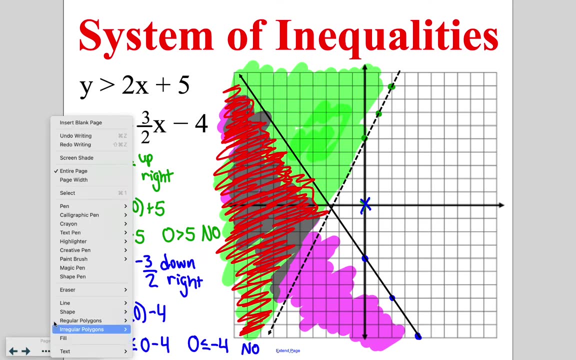 where these two overlap. so your first option is to take a third color or take your pencil and make it much darker where these two overlap. so that's our first option. the other option: if you prefer, you can go back and erase the parts where they do not overlap. so you could have erased all of this up here, because 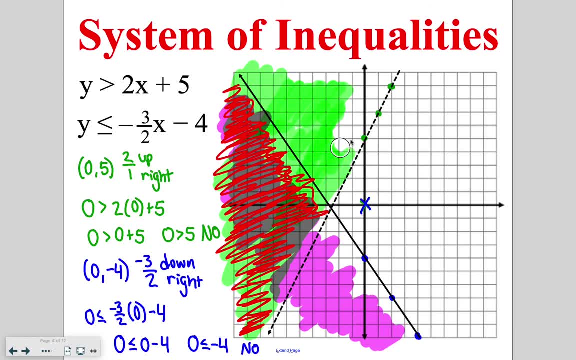 this only works for a particular color type, so if we do this, we would have to do this from either this in the right hand corner or the left hand. this is my right-hand section, so that's our first option and thentu for the first line, a little bit more difficult for me to erase on the computer because it 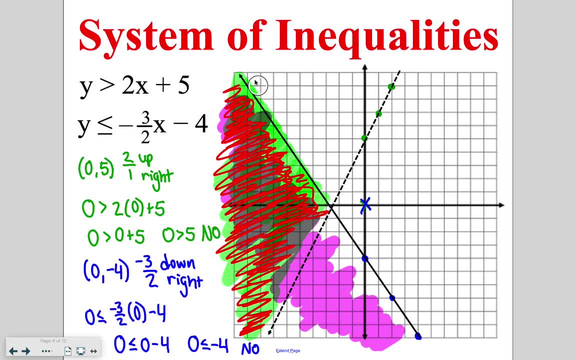 won't let me get super close, but everything that is on the opposite side of this line should be gone, and then we would also have to erase everything that would be not in the overlap for the other line. so again, you have the two options. you can either color in the 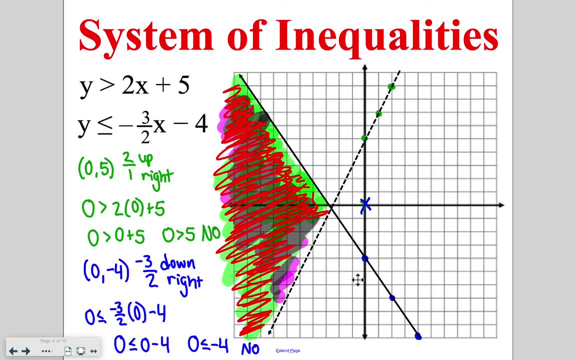 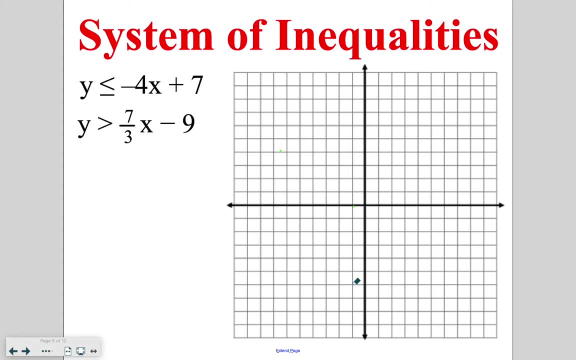 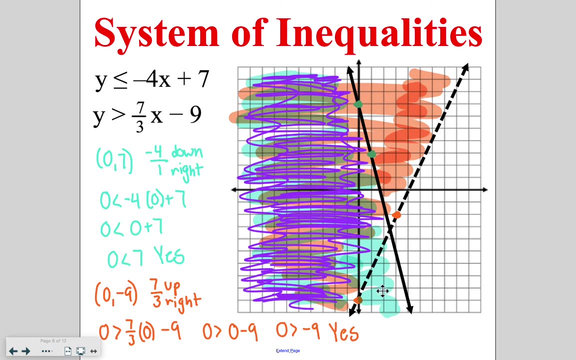 area darker, or you could erase to get rid of the pieces that do not overlap. go ahead and try this one on your own. so the first graph is shown in the light blue here, or the light green. the second graph is shown in the orange. this is an example of what it would. 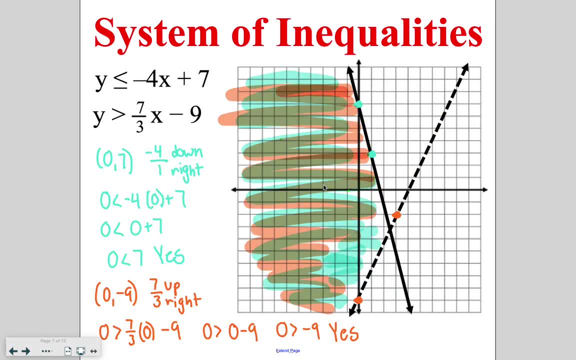 look like if you highlighted the overlap, if you preferred to erase and just eliminate those two pieces that do not overlap, it would look like this once again: anything in that highlighted area, whether it's shaded darker or whether it's erased, anything in that area is a solution. 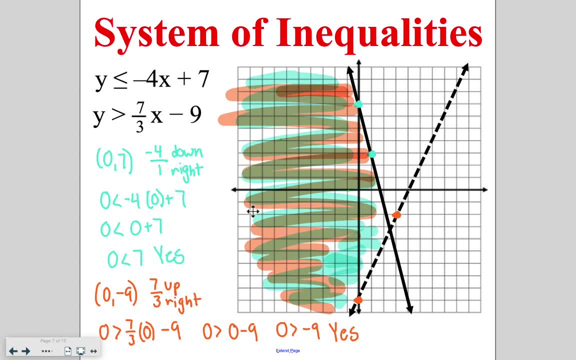 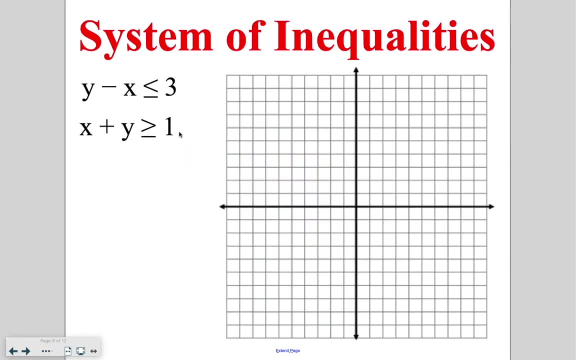 to both problems, which is what we are looking for. so any coordinate pair that lies in this highlighted area is a solution to both problems. once again, sometimes we have problems that are not in y equals mx plus b format, so we are going to have to fix those. so i'm going to start by fixing the first one in order to get y by itself. 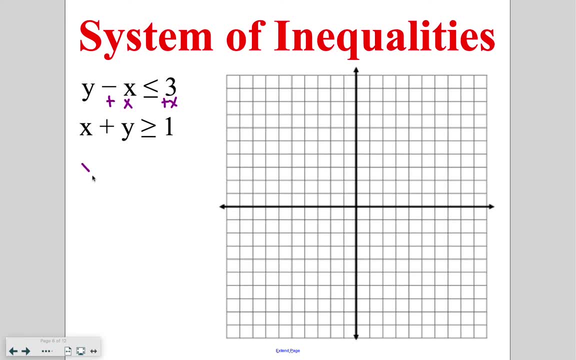 i'm going to add x to both sides, so my new equation becomes: y is less than or equal to x plus three. going ahead and picking out my y intercept, i'm at zero three. picking out my slope, which is one, i'm going to make that one over one as a fraction. so up one and over. 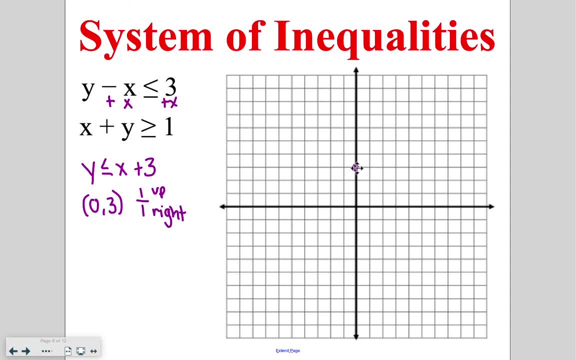 one. so i go zero, one, two, three on my graph, up one and over one, and you can repeat that process up one and over one again. i have an equal to sign in my inequality. so that means i am going to use a solid line as i fill this in and when i 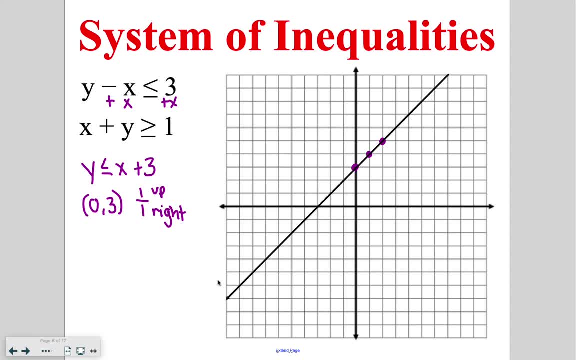 graph. i'm going to end up with this line right here. i still need to plug in my test point once again. i'm going to pick zero, zero. when i do that, i'm going to plug it back into my original function. so zero is less than or equal to three, giving me the statement: zero is less than or equal to three. 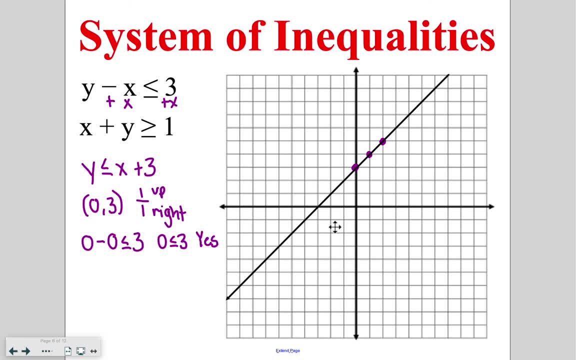 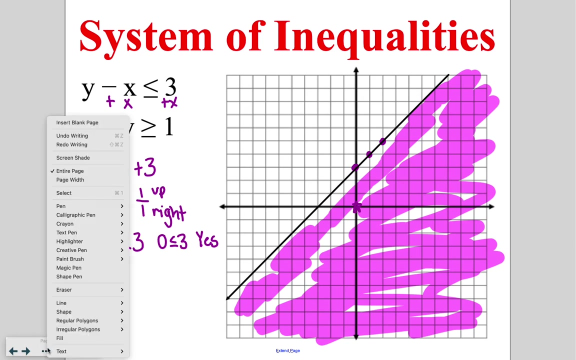 which is going to be a true statement. so that means zero. zero is included for this first inequality. so i'm going to highlight to the right of this line, which is going to give me everything over here. then i once again need to rearrange my equation, so i'm going to go ahead and in this case, subtract x from both. 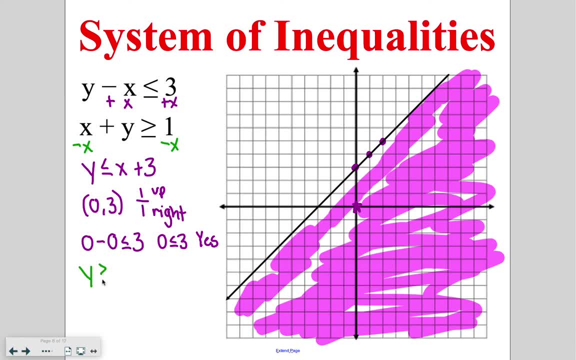 sides. so my new inequality says y is greater than or equal to negative x plus one. picking out my y intercept, i've got zero one and my slope now is negative one or negative one over one, meaning that i'm going to go down one and right one. so i'm going to put my initial y intercept at zero and i'm going to 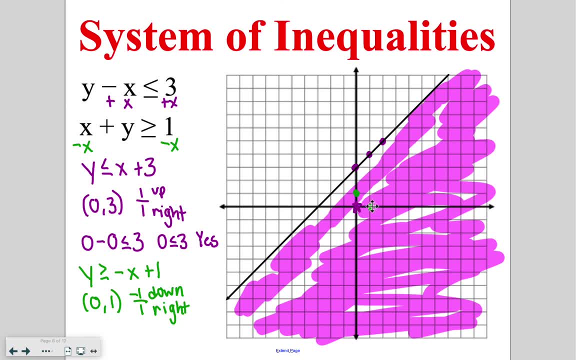 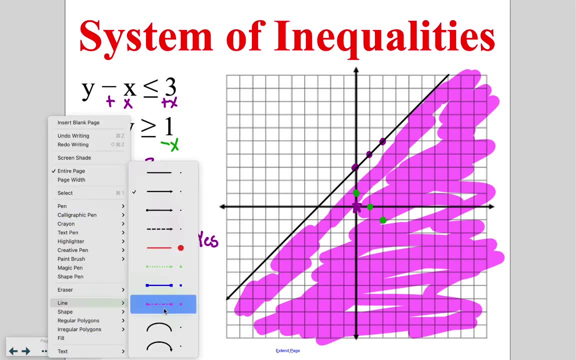 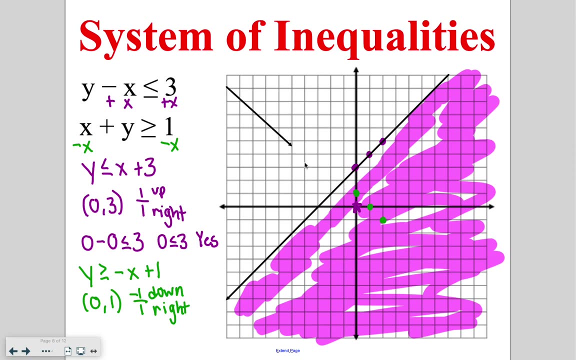 subtract at up one, and then i'm going to go down one and over one, and i can repeat the process of down one and over one. once again, i have an equal sign in my inequality. so that means i am going to use a solid line and as i do this, when i put my line onto my graph, i'm going to fix that a little. 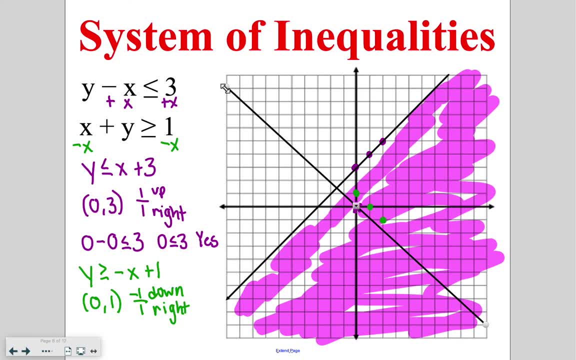 bit. i missed my points, so bear with me. i'm going to put my line through my points and i end up right here. once again, i need to plug in a test point. plugging into my original equation. i'm going to have zero plus zero is greater than or equal to one, giving me the statement that zero is greater. 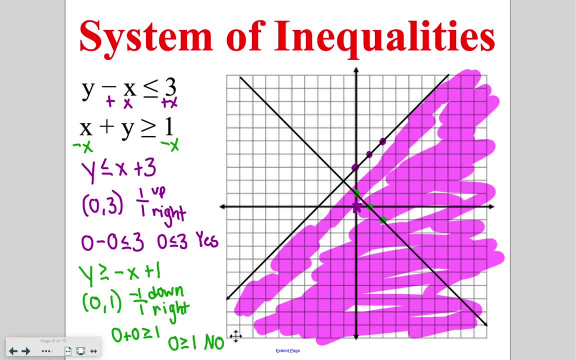 than or equal to one. this is a false statement. so for my second, inequality: zero, zero is not included, so i'm going to go on the opposite side of that line, which is going to be everything on this right side, as i am highlighting. so everything over here. once again, you have the 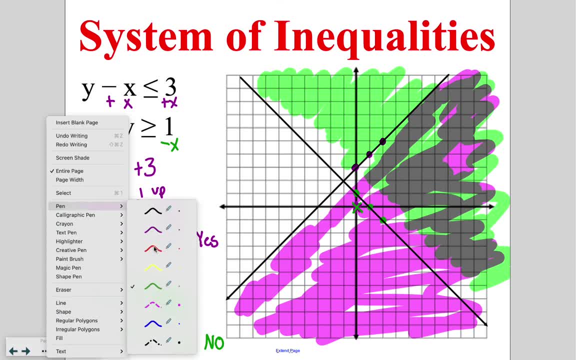 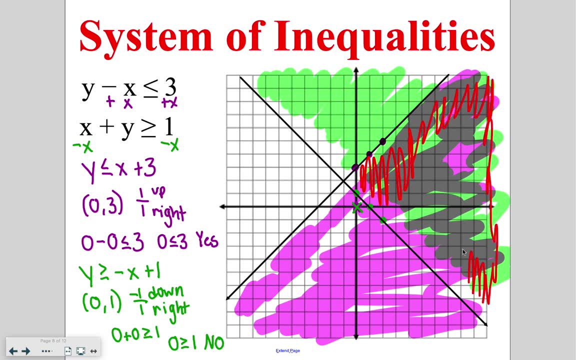 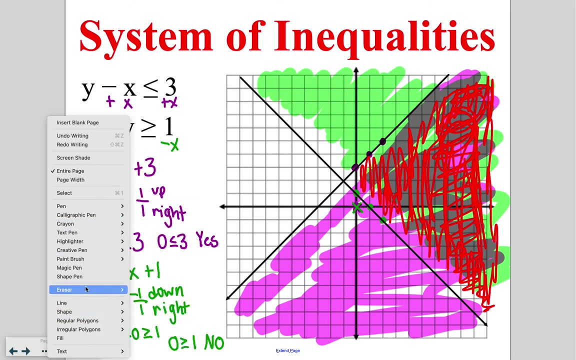 option now to either make the overlap area darker so i could take my pencil or a third color if you wanted to do this- with color and shade in this area darker, so that i know everything in this particular area is going to be a solution to my problem, or, once again. your second option is to go through and erase anything outside of that. 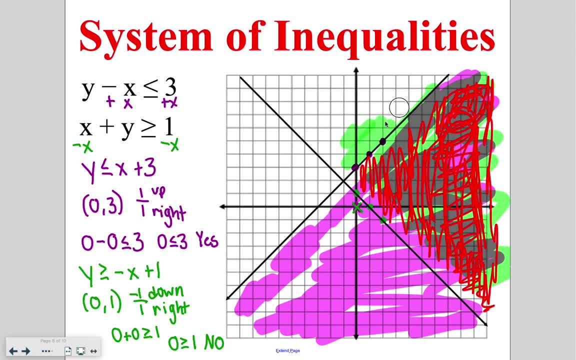 overlap. so if you preferred to erase, i would erase all of this for my second equation and everything down here for my first equation. so again you have the option about whether you want to highlight that overlap. again, a little bit more difficult for me to erase this highlighter on the computer. i don't want to erase my points, but everything. 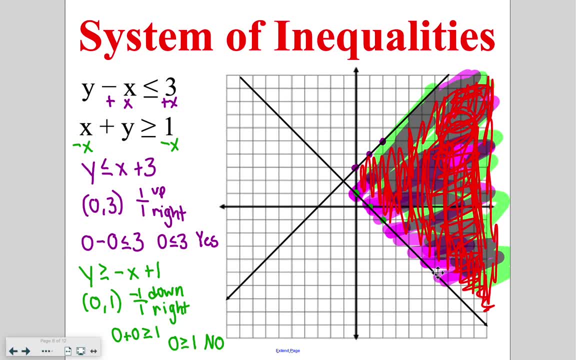 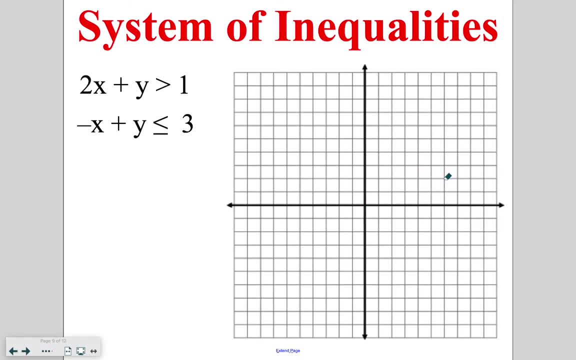 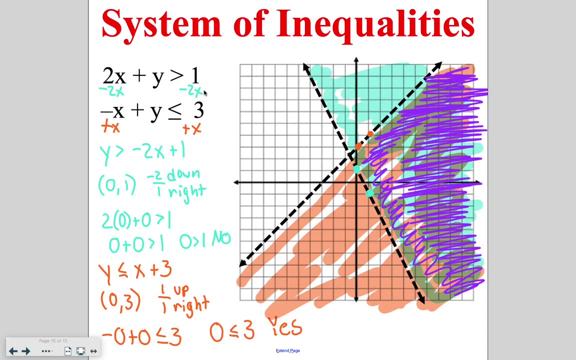 over here should be erased. if you are going with that eraser method- or you can highlight everything by making it darker- go ahead and try this one on your own. first one, rearranging by subtracting to x, picking out your y intercept and your slope, and then, when you plug in zero, zero it's going to give. 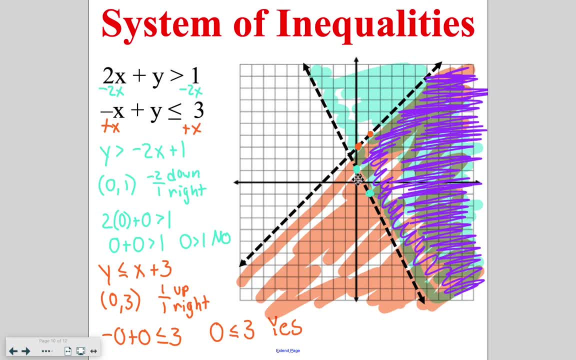 you a plus statement. so we are going to the right of that line, since zero, zero was on the left. the second one: we're going to add x to both sides. giving you y is less than or equal to x plus three, plugging in zero, zero. this time we end up with a true statement. so everything that was on the right. 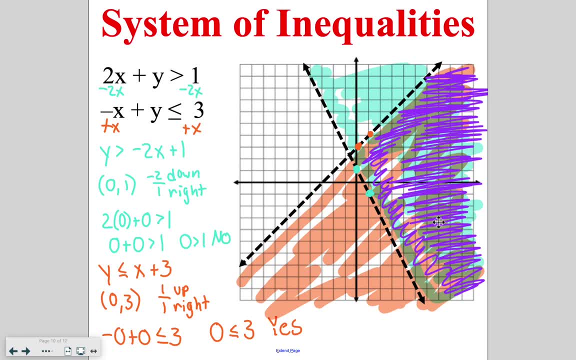 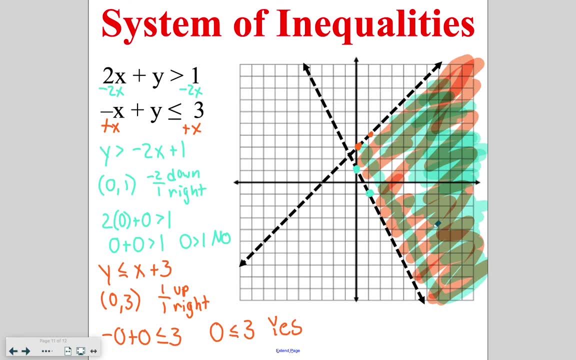 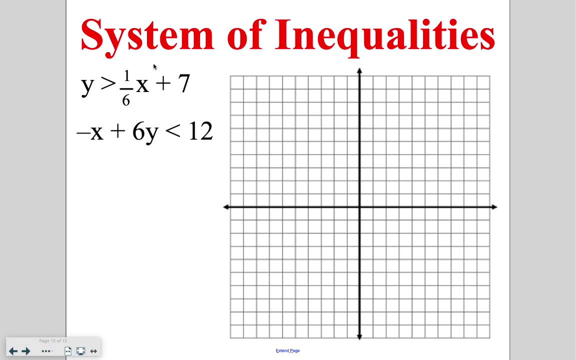 side of that line is true. right here i have it shown, where i highlighted that area of overlap to make it darker and left the other pieces. here is what it would look like if you preferred that way. so i'm going to go back to the eraser method. one last example i want to go through here. 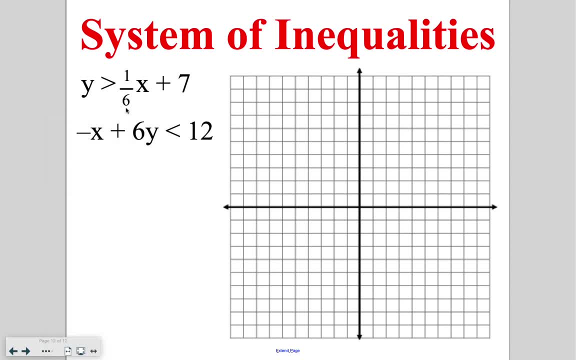 in this first one we are already in y equals mx plus b format, so i can pick out my y-intercept, which is going to be 0- 7, and my slope of 1- 6 tells me to go up 1 and to the right, 6. so i'm going to go. 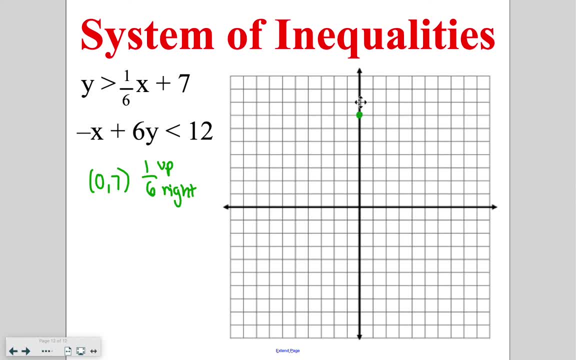 0, 1, 2, 3, 4, 5, 6, 7 up, and then up 1 and over 1, 2, two, three, four, five, six. if i go up and over again, that doesn't fit on my graph. so if you would, 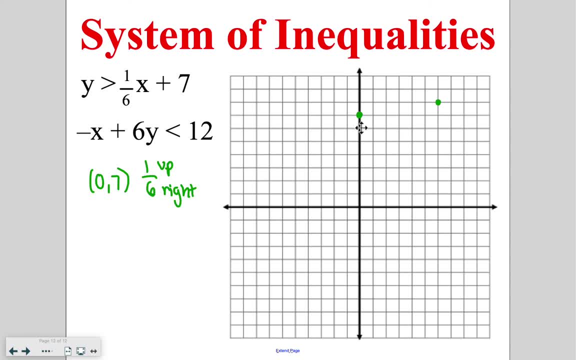 prefer to add a third point going opposite. so down one and then left one, two, three, four, five, six would let you complete that i do not have an equal sign in my inequality, so i am going to put a dashed line onto my graph and i've got it going through the points i'm going to have to adjust. 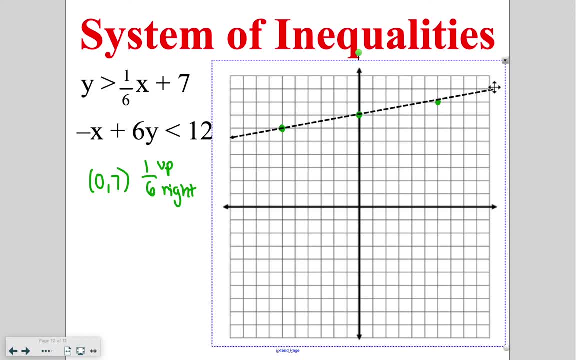 this because i am on the computer, so i'm going to take this and adjust it down a little bit so i have my line through my three points once again. then i need to put in a test point to decide which side to shade i'm going to plug in: zero, zero. so zero is greater than one, six times zero plus. 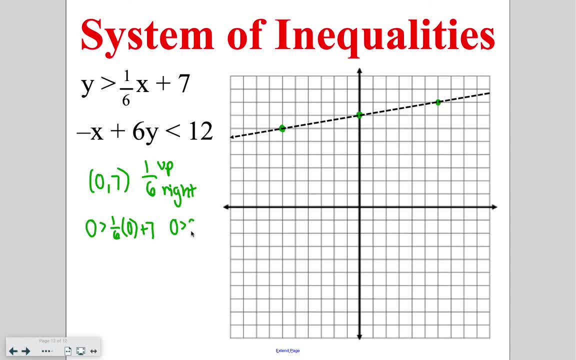 seven, giving me the statement zero is greater than zero plus seven or zero is greater than seven, which is a false statement. so i do not include zero, zero in my answer, which means when i highlight, i'm going to go above this line. so i've got everything above. 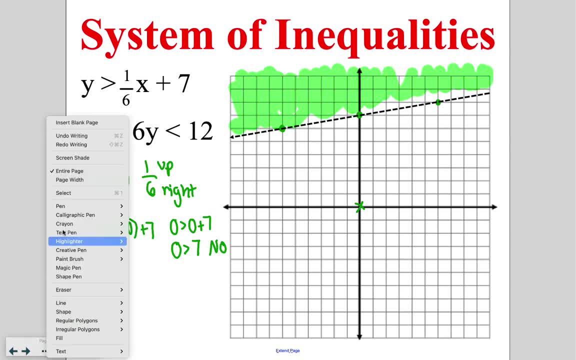 this line as part of my solution for the second equation. i do need to do some rearranging, because y is not by itself. my first step, then, is going to be to add x to both sides, giving me y is less than x plus 12.. then i need to divide everything by six, remembering that there used to 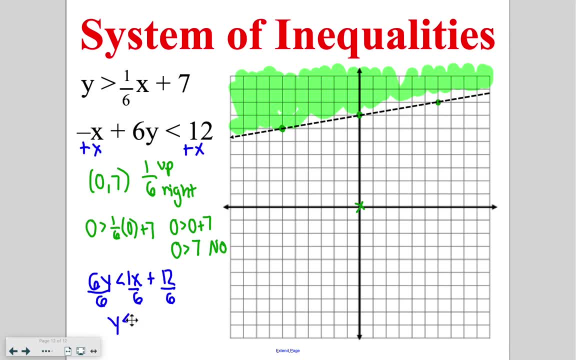 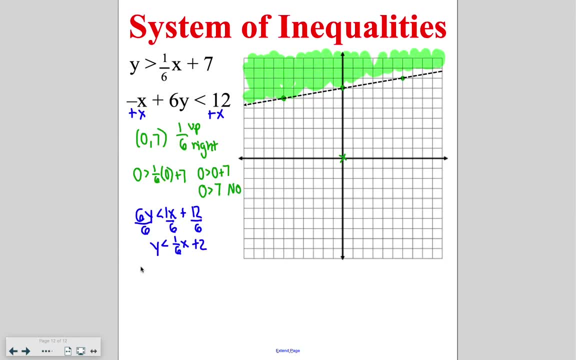 be a one in front of the x. so i've got y is less than one sixth, x plus two. as i pull out my uh y intercept, i've got zero two and my slope once again of one sixth is going to be up one and right six. so i start at zero one, two this time. going up one, one, two, three, four. 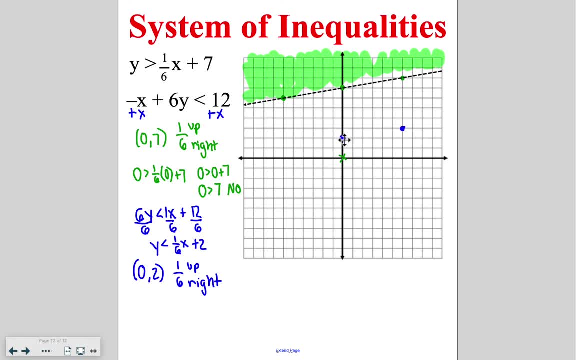 five, six to the right, and then i have to go opposite. so down one and then left six, if i wanted to put that second point on there. once again, no equal sign in that inequality. so i'm going to go once again with a dashed line and i've got that going through my points.